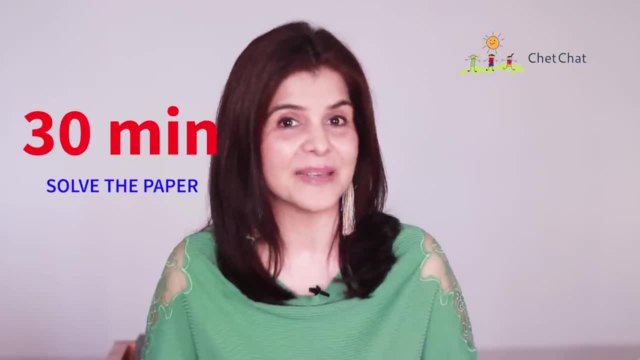 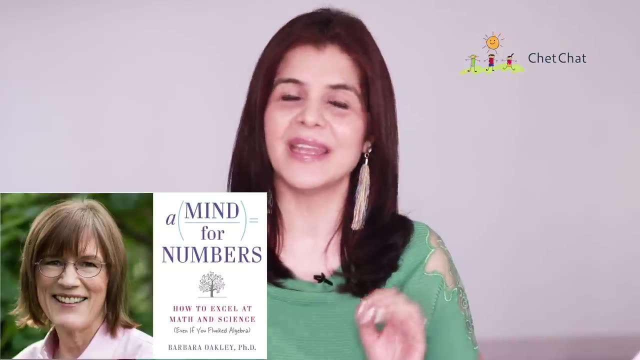 And this will give you an initial boost of confidence. The next 30 minutes go through the rest of the questions. If something is very hard, don't spend more than one minute on it. In her book, A Mind for Numbers, Barbara Oakley recommends the hard start. 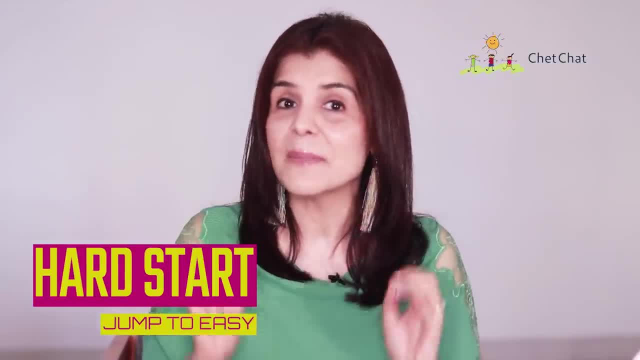 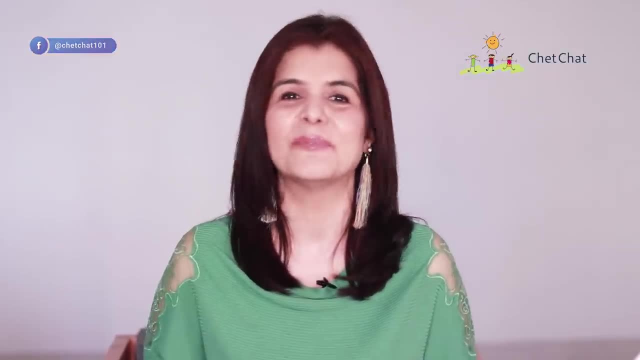 jump to easy technique, where she says that as soon as you hit a mental roadblock, shift gears and get to work on easier questions. The brain is a powerful organ. It keeps working in the background. Also, you might get some clues in some other questions. 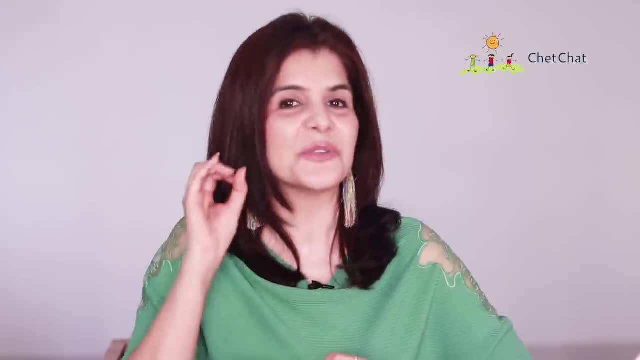 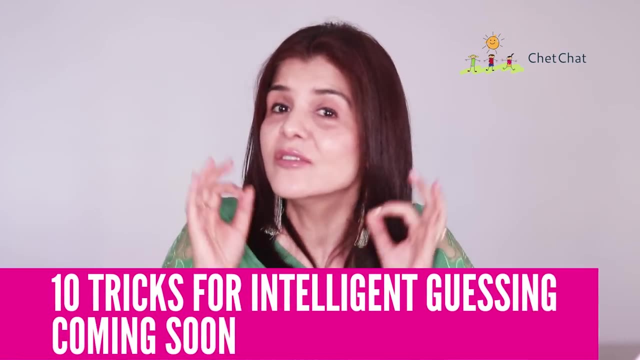 And the last 15 minutes. this is the time to tackle those challenging problems and perhaps make some intelligent guesses for those no go questions, And we have 10 super tricks for that coming up later on in this video. Hey, before I give you strategy number two, 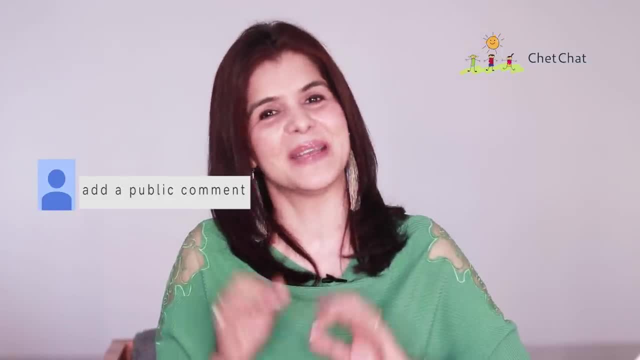 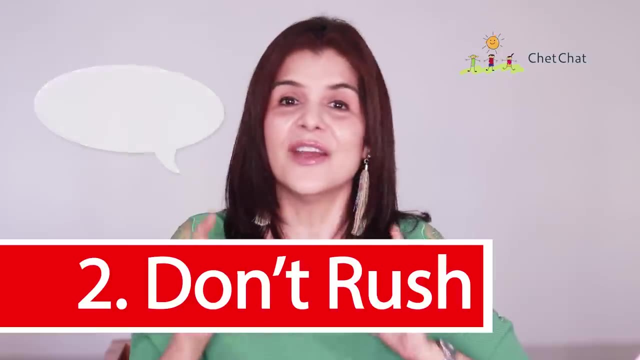 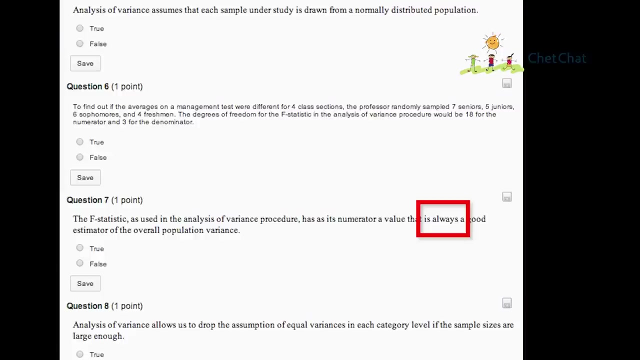 if you want a shout out in my next video, write me a catchy comment with the hashtag Chedd Chatters. Strategy number 2, don't rush. Read the question twice. Pay attention to words like NOT always, which completely change the question. 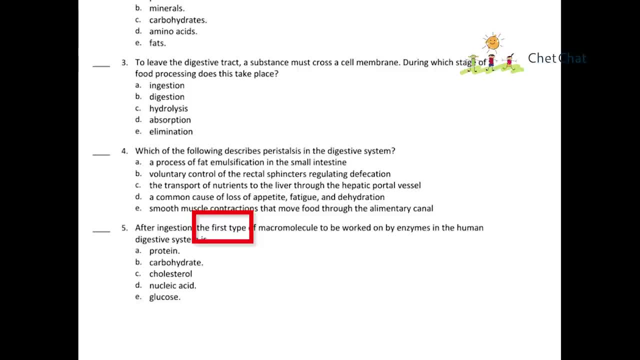 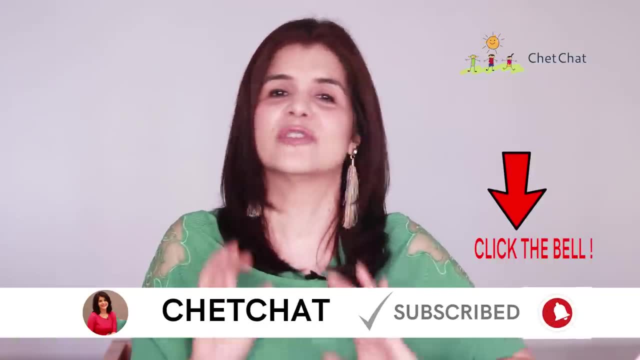 Also double check the exact requirements of the question. underline these words and other important keywords. If you think the first option is correct, don't rush to circle the OMR sheet. Make sure you read all the options carefully before choosing the answer. 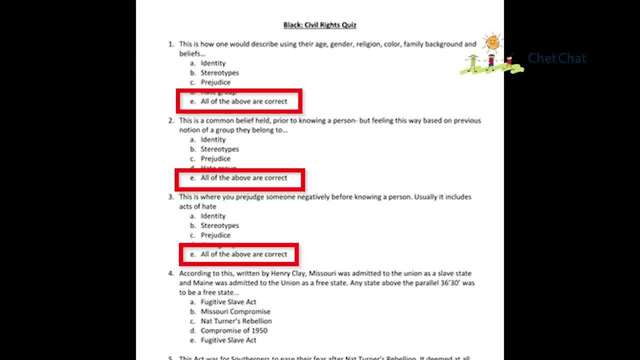 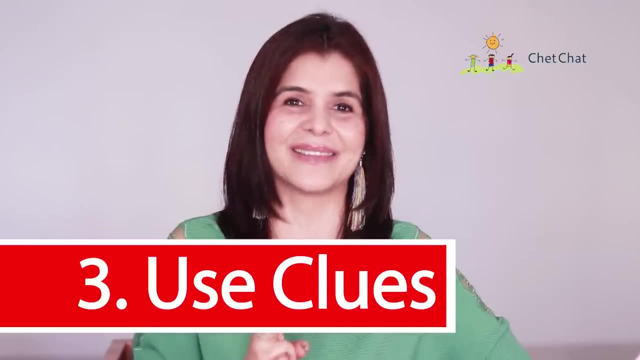 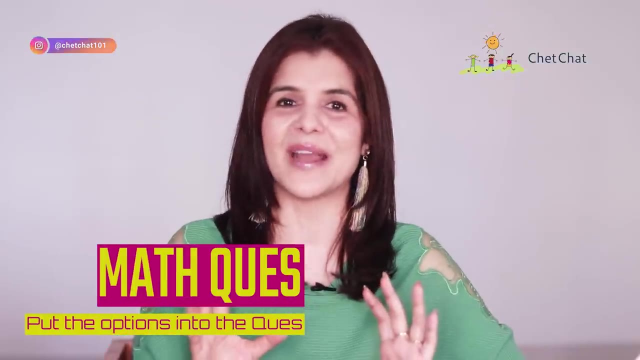 never know you might find- and all of the above somewhere. strategy number three: use clues from the question. this strategy has three sub parts, haha, just like MCQs. first, in math questions, if the calculation seems too long-winded, one easy method is to put the options back into the question and check if the 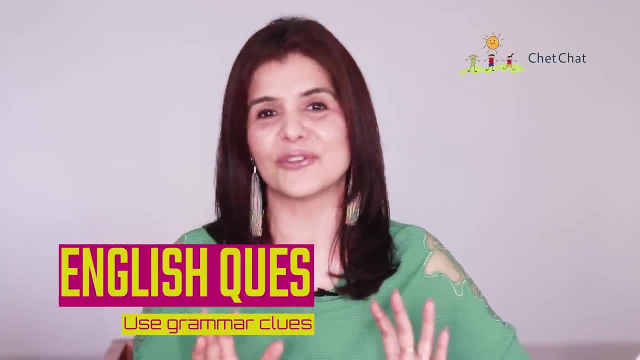 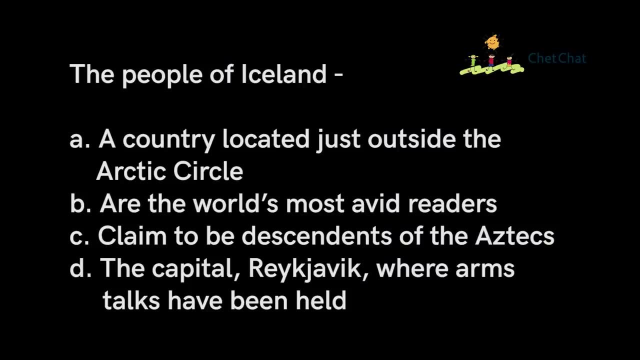 equation balances two in English or social studies based questions. use grammar as a tool to help you. example: this is your question. option a is missing the verb and option D has no connection to the people of Iceland. these options can be eliminated, even though both may be true and you're. 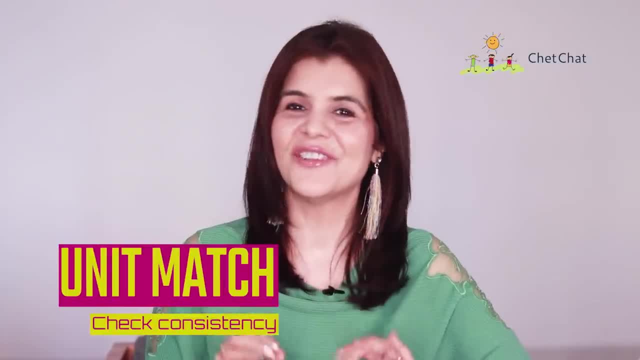 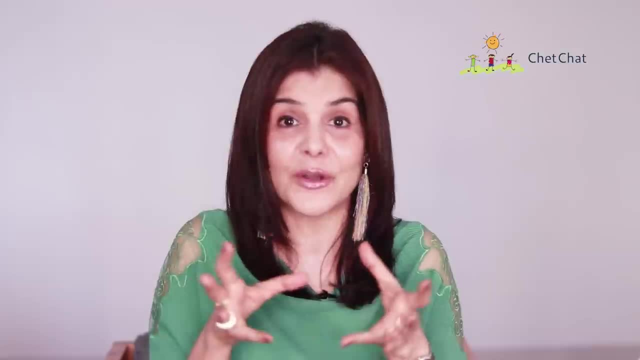 finally left with option B and C, three check units and dimensions. these will give you vital clues. so if the calculation is for an area of an object, for example, rule out the options that are not inscribed in the question. so if the calculation is for an area of an object, 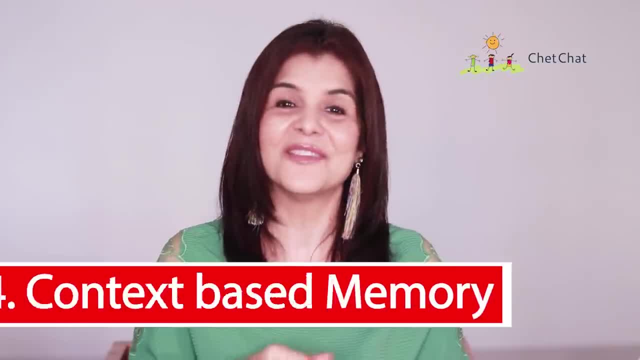 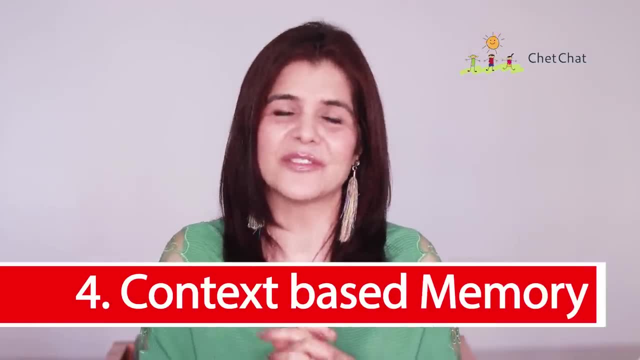 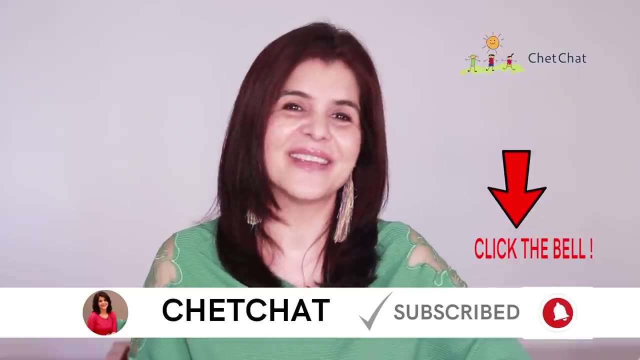 and there are no possible answers. you have to build two square units even before you begin to solve the question. strategy number four is called context-based memory. sometimes we ponder over MCQ questions with foggy answers in our mind. we trying a level best to recall it, but you're just stuck and to 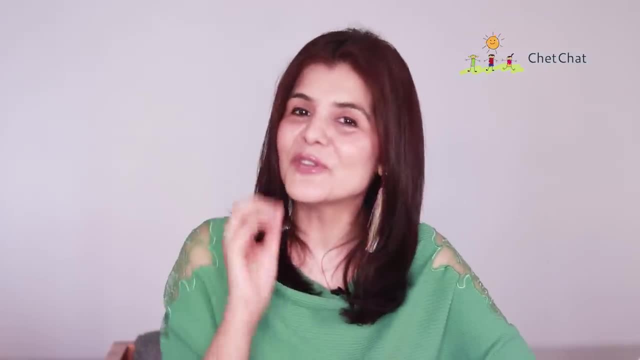 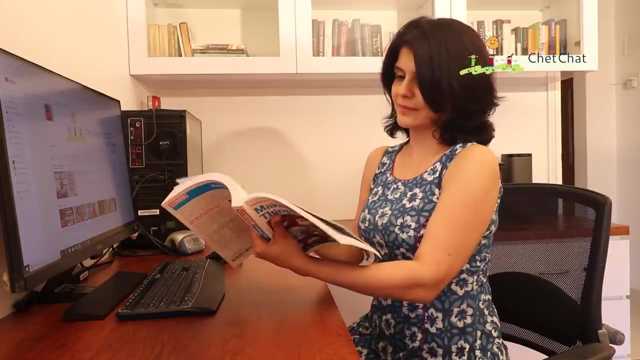 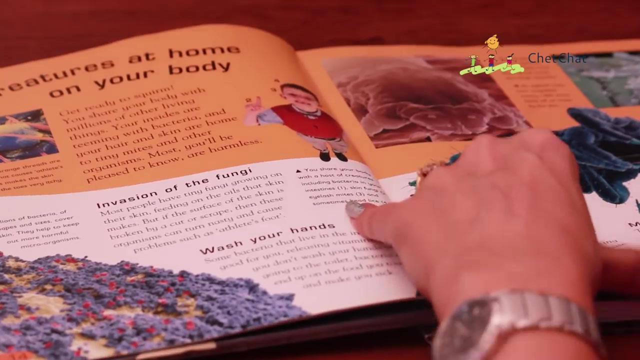 our rescue. psychology has a trick called context-based memory. it says that to recall some missing information, try to remember where you studied that piece of- in a book or online. was it from a tuition teacher or from a friend? even trying to remember which corner of the page that graph was, that may trigger your mind to connect the dots and find the missing. 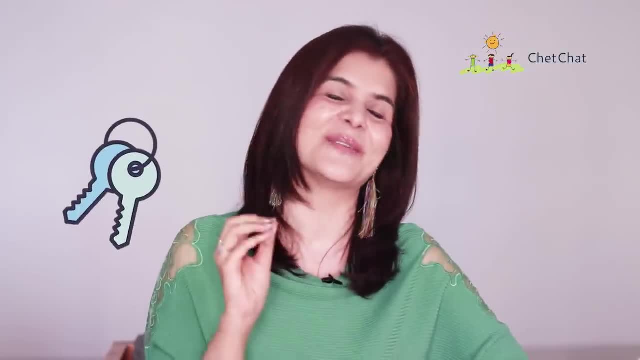 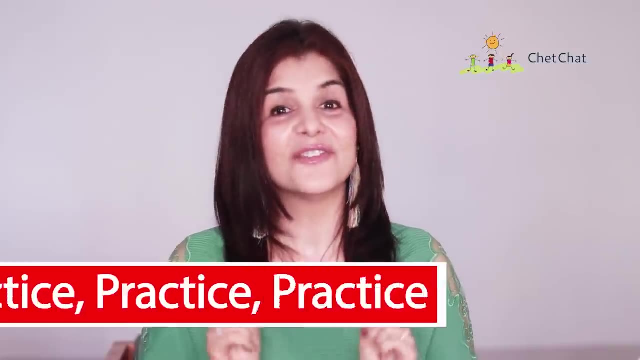 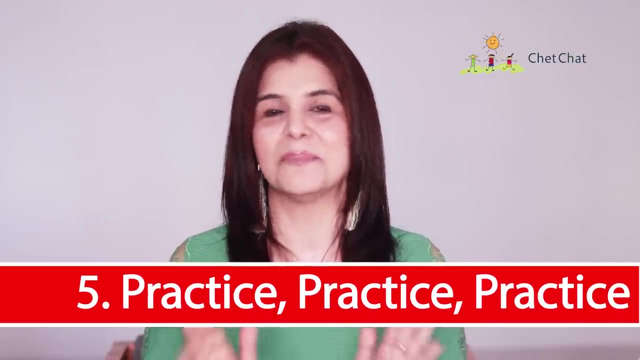 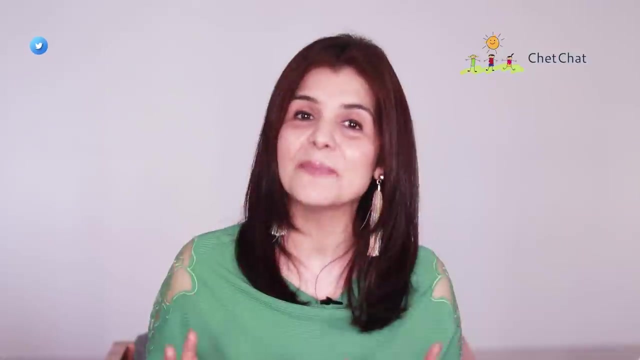 information. it works, even if you forgot where you kept your keys. and with that key information, let's move on to our next strategy. strategy number five is practice, practice, practice. there is no strategy to crack mcqs that beats this one. practice every day, check your answers, go back to the concepts and understand the types of questions being asked. and if you want a perfect 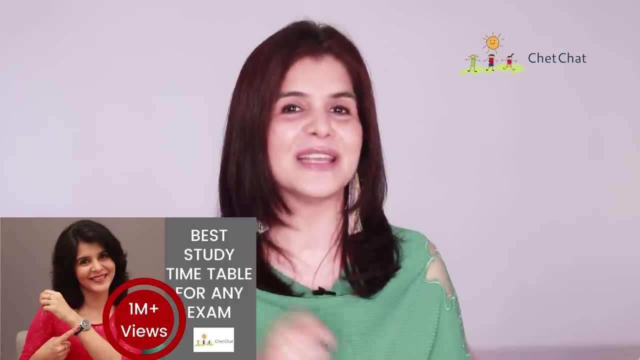 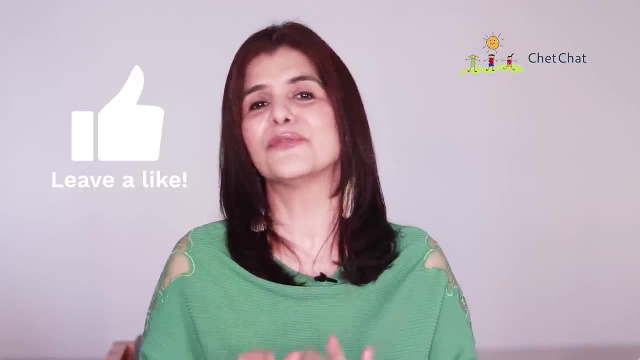 timetable, perhaps to study for any exam- then i will drop a link for you under this video, and if you're enjoying this, then don't forget to press that little thumbs up. now you're left with the tough questions, and if there is no negative marking- or maybe the negative marking is very 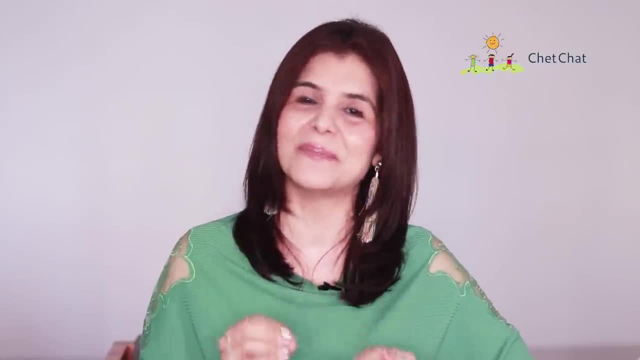 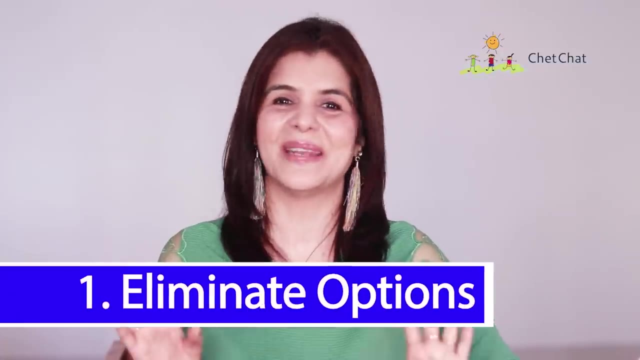 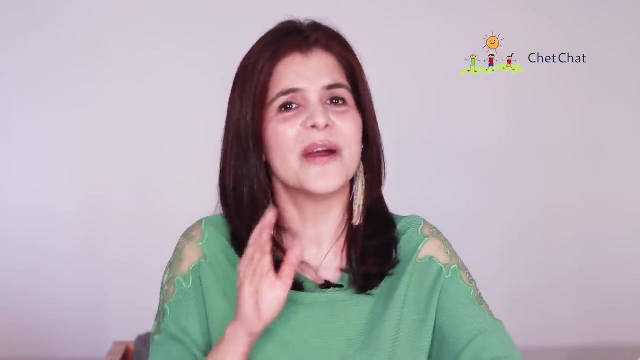 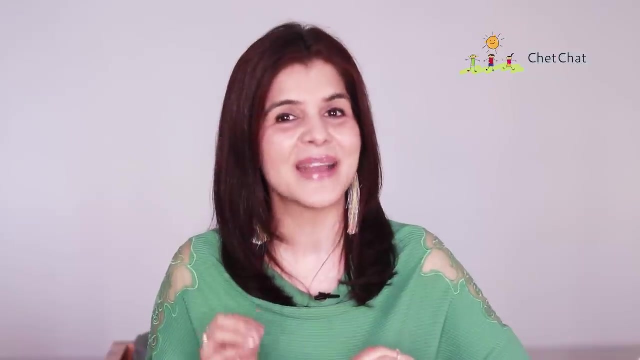 low, then perhaps you can go ahead and make some smart guesses. so here are my 10 tricks for intelligent guessing. tip number one: eliminate the options. the general formula for solving mcq is to increase the probability of the right answer by removing all the possible wrong answers. to start by removing the options which are clearly wrong. sometimes you might get lucky. 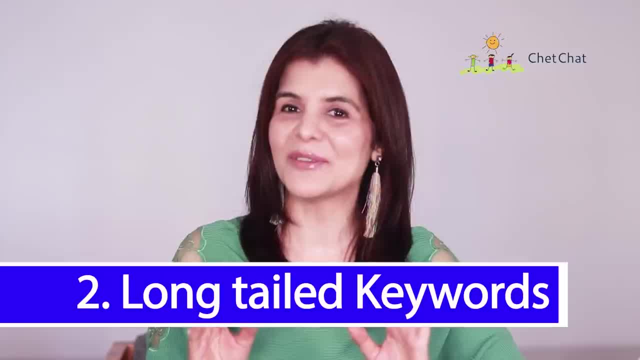 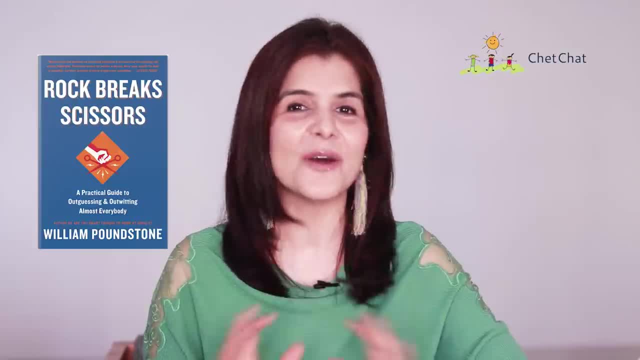 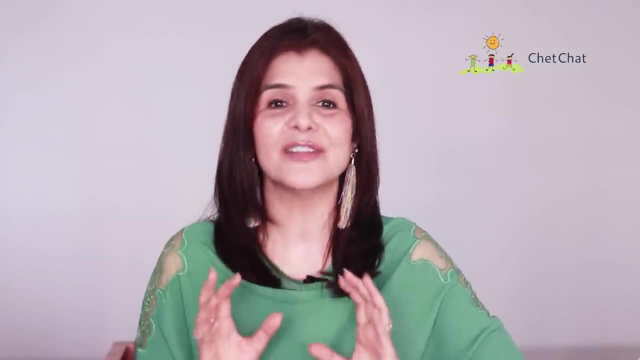 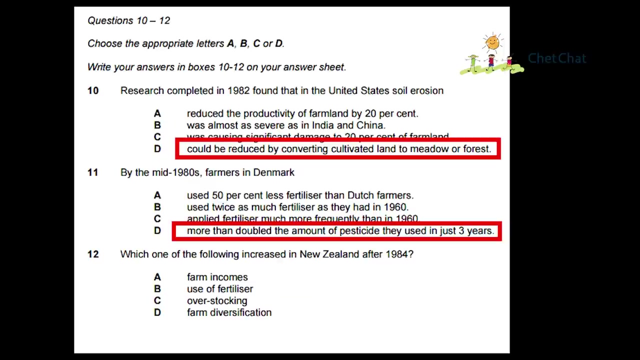 and be left with only one option. tip number two long tail keywords in his book rock break scissors: a practical guide to out guessing and outwitting almost everybody. the author william poundstone has revealed some marvelous findings through his research with huge sets of mcq data. his book reveals that the option with the longest statement. 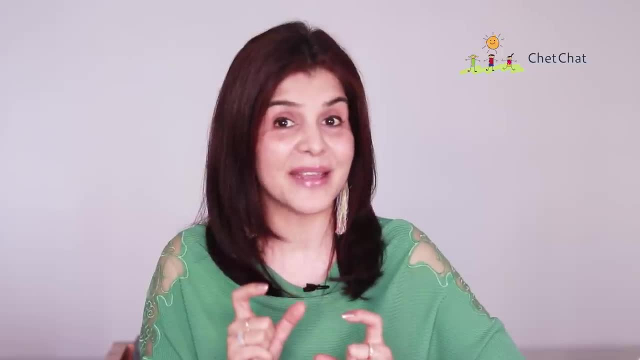 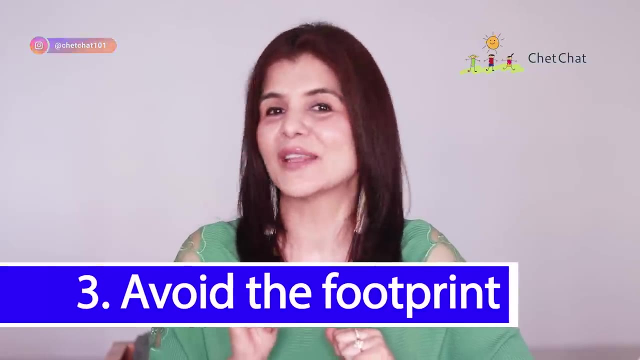 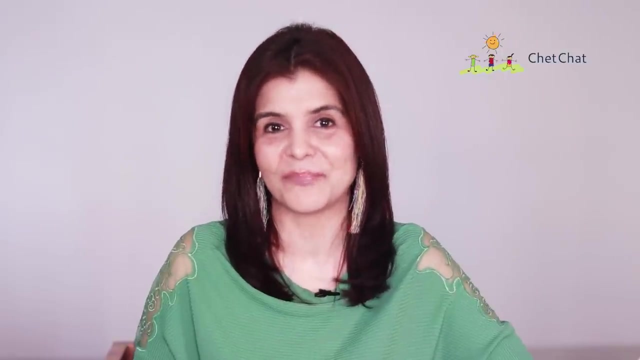 has the highest probability of being right, because the test makers have to make sure that the right answer is indisputably right. tip number three: avoid the footprint. poundstone also discovered that two successive questions rarely have the same correct option. for example, if you're solving question number 30 and find 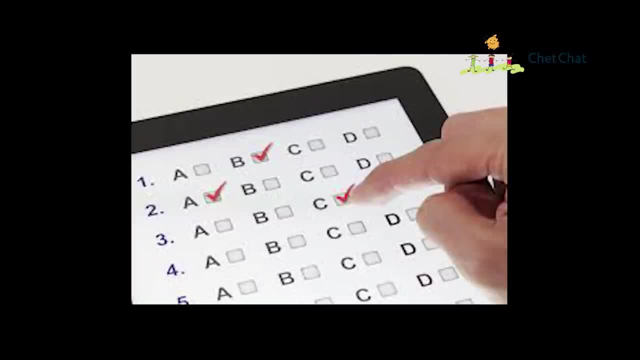 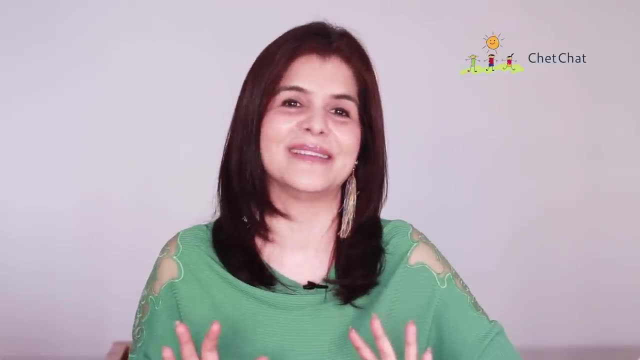 yourself clueless, then look at the answer to question number 29 and question number 31 and don't select the same letters. they have the least probability of being correct. tip number four: golden options. research has shown that the answer to the question number 29 and the question number 31 is the. 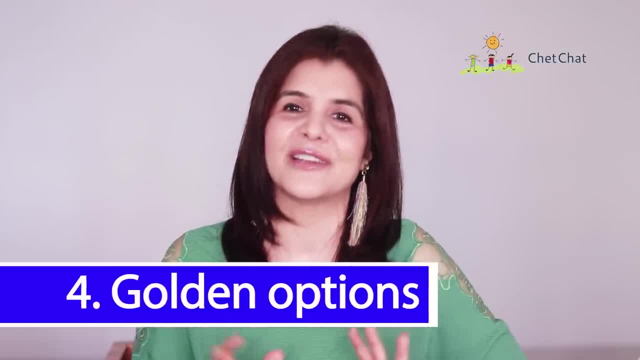 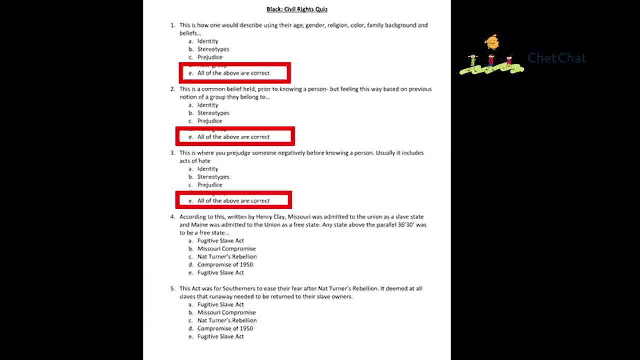 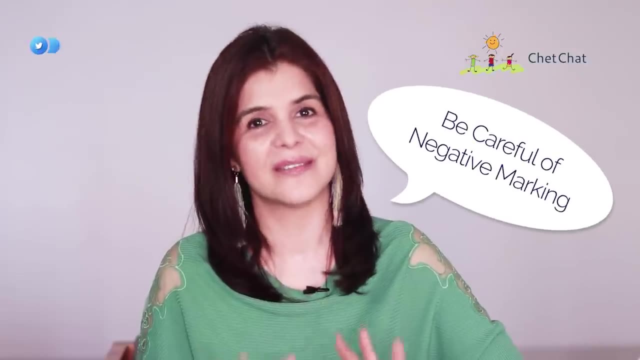 shown that if you don't know the answer at all for any particular mcq question and one of the options has either all of the above or none of the above, you can bet on these options. they have a disproportionately high probability of being correct. one reminder, however, is to make sure. 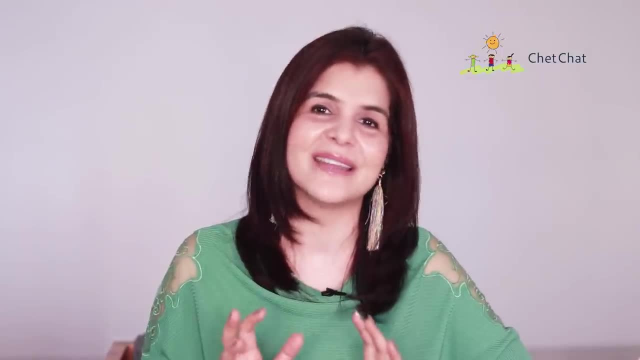 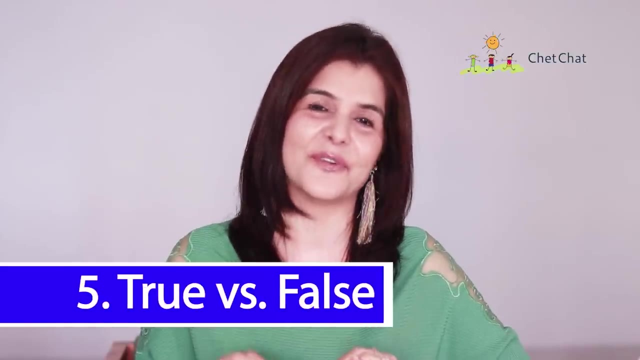 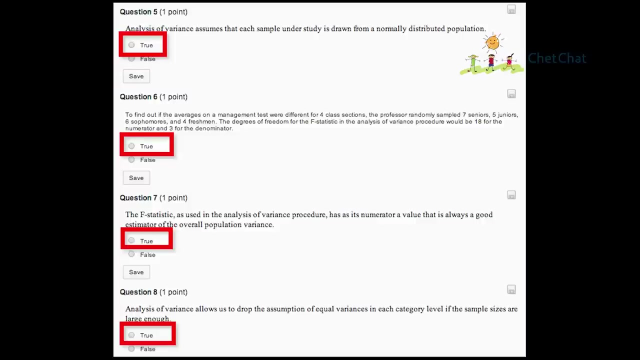 that either there is no negative marking in your paper or the negative marking is very low. before you try guessing too many answers. tip number five: true versus false. in the tug of war between true and false in a true false question, poundstone revealed that true is more likely to be the. 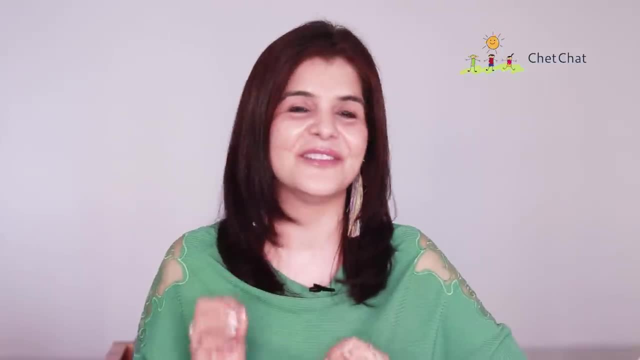 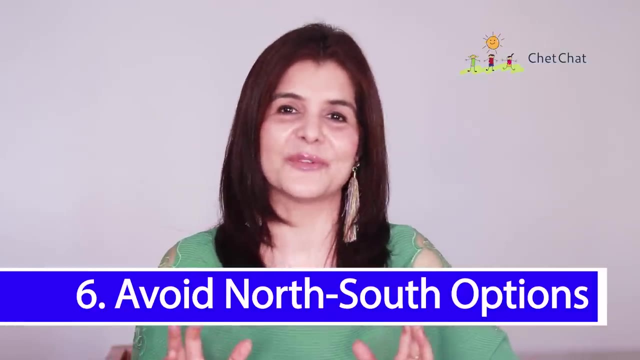 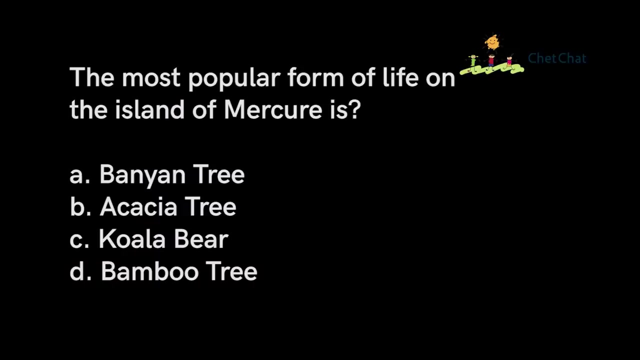 correct answer than false. so if you're guessing wildly, then choose true tip number six. avoid north south options, remove extreme values or completely unrelated values. for example, you have four options, like banyan tree, acacia tree, koala bear and bamboo tree. clearly koala bear would be the wrong answer. similarly with numbers. 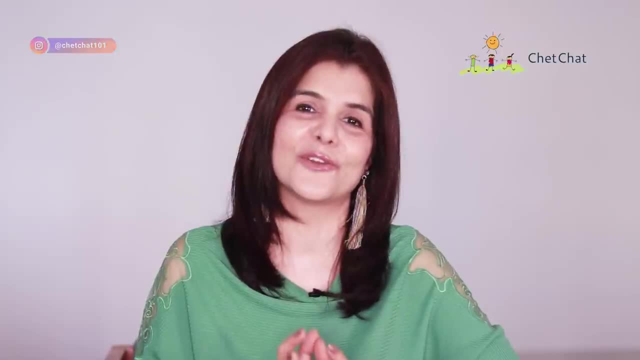 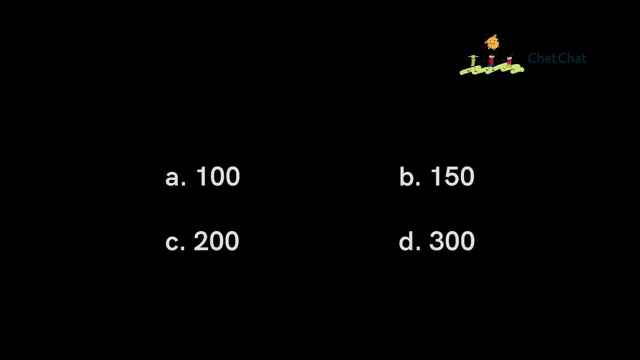 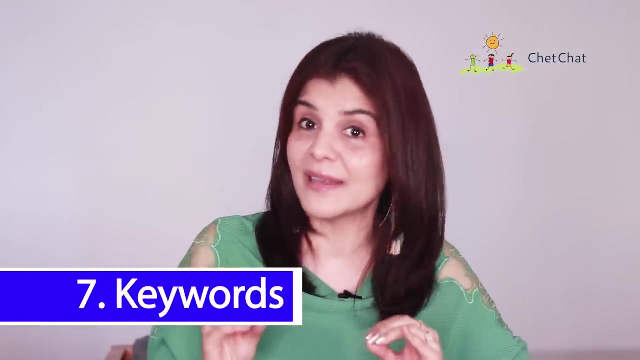 remove extreme numbers when in doubt. the middle order options are much safer. for example, if your options are 100, 150, 200 and 300, then perhaps 300 may not be the right answer. tip number seven: if two options are similar sounding or if they have the same keyword appearing in both these options.